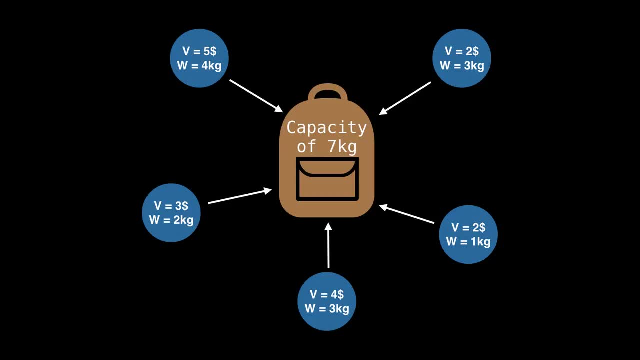 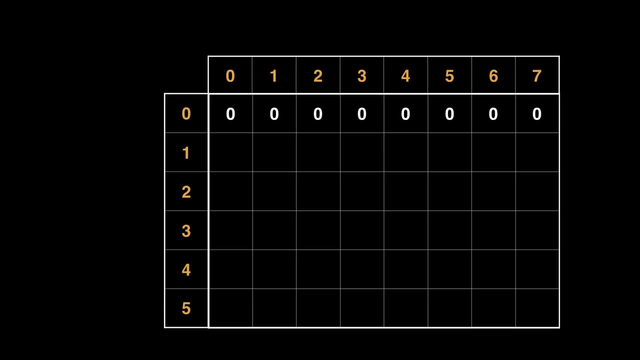 to pick. So let's see how we can solve this problem with dynamic programming. The first thing we'll need is a table of values to store various states. In the context of a knapsack problem, we can think of a row in this table as representing. 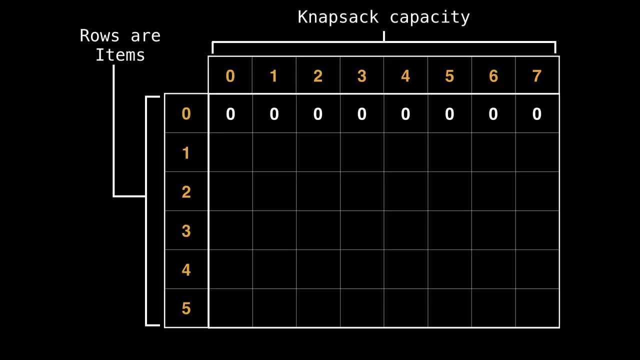 an individual item and the columns as representing various capacities or maximum capacities are knapsack can have. So how we're going to solve the knapsack problem is going to be by considering the first item and then figuring out all the best possible values we can achieve for each. 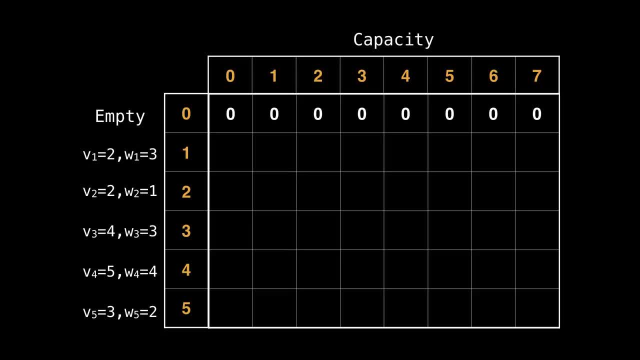 capacity, And then after that, considering the second item and reusing information we know from the first item, to formulate a combined best value for those two items and then incorporating a third and a fourth item and etc. What we want to do for each column in the current 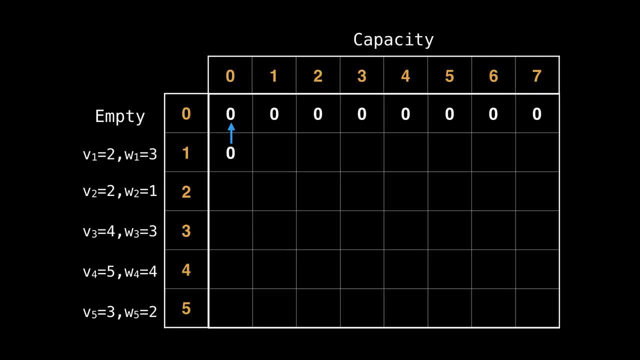 row is figure out if we should or should not include the current item. If we don't include the current item, then we look one row above. But if we do include the current item, then we still look one row above, but shifted over by the weight of the current item, because 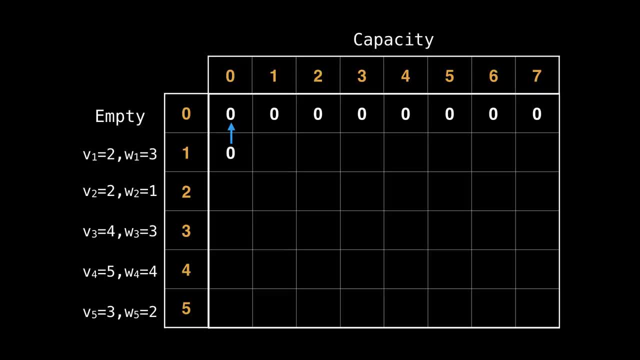 that would be the state with the best possible value and a knapsack large enough to hold our item. Right now. item one has a value of two and a weight of three. The weight of three does not fit within a knapsack of capacity zero, So the best we can do is have an empty. 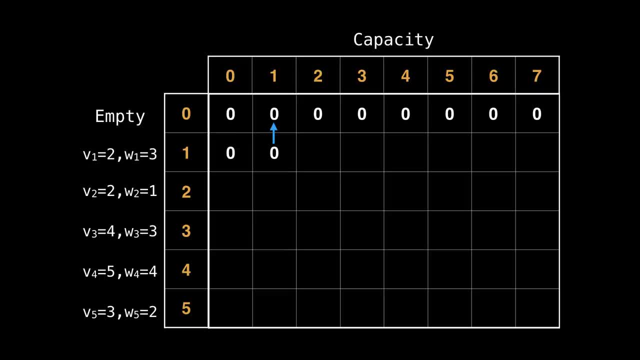 knapsack of value zero. Similarly for capacity of one And a capacity of two, but capacity three. we have enough room to fit item one. notice that there are now two arrows. the short arrow points to the row above us, which represents 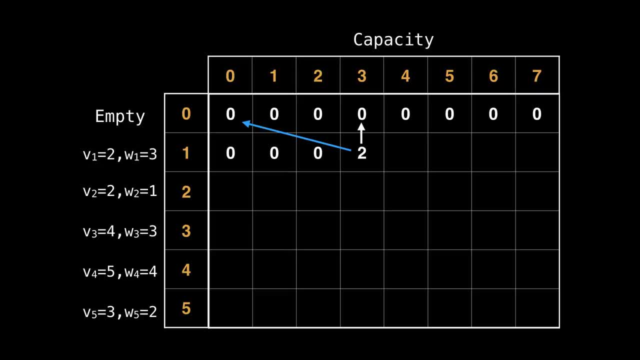 the state of not including the current item and taking the best value from before, which, in this case, is zero. the longer arrow points the state in which we can include item one and add its value to the new state. In this case, that is two, because item one has a. 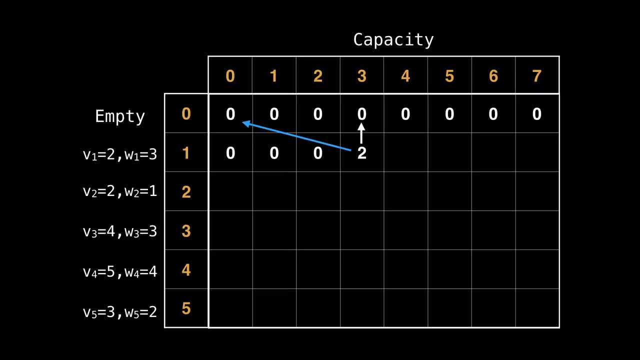 value. Value of two. because the next state always needs to include or not include the current item, I will label the arrow which yields the best value for the next cell to be blue. So keep your attention focused on the blue arrows to know which of the previous states. 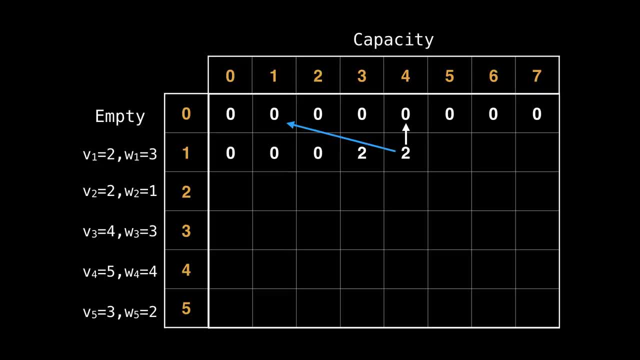 best contributed to the new state. Moving along, you can see that we increase the capacity And we are still able to include item one, as we did before. This is because the size of our knapsack keeps increasing, So this makes sense. So the rest of this row. 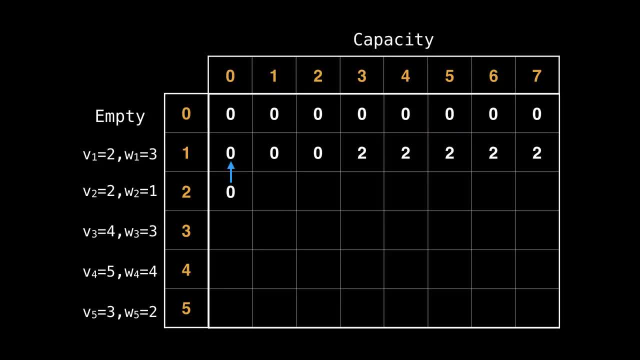 will continue to have a value two when we get to the next item. our column is zero, So our capacity is zero and we're not able to include any items, So we get a value of zero right here Next up. if we consider a knapsack of capacity, one item two fits into. 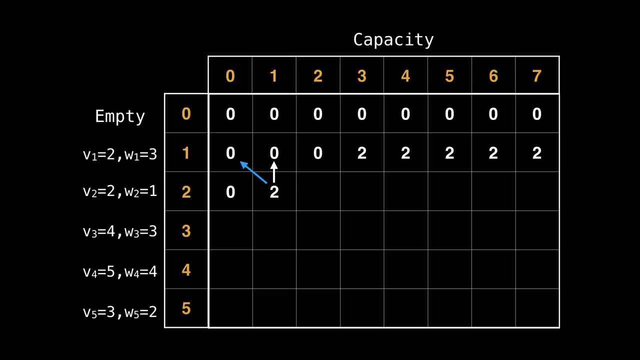 this knapsack so we can include it, Giving us a value of two in the cell. Moving along, we can also include item two for a capacity of two. Now, something interesting happens: when we consider a knapsack, of capacity three, we can either get a value of two from picking item one. this is the state directly. 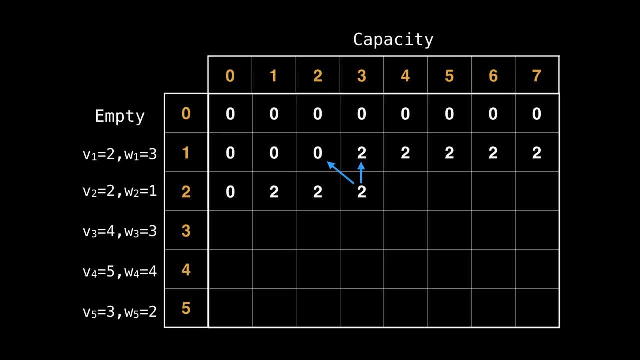 above us, or we can equivalently get a value of two by selecting item two with the diagonal arrow. So there is a tie and in either case we'll get a best value To this. next date is also particularly interesting. We've increased the capacity of our knapsack. 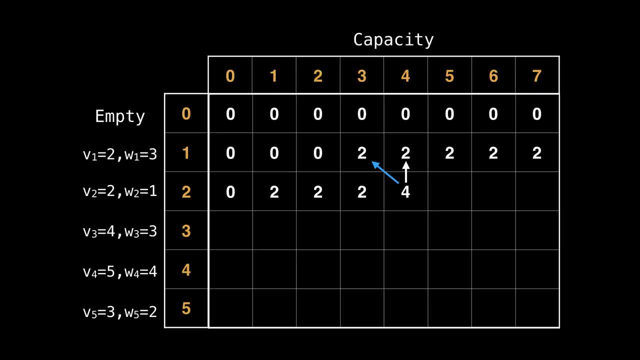 to four. So we're able to fit both item one and item two into the knapsack, giving us a best value of four. This pattern continues on for the next couple cells When we introduce item three. for the first few knapsack capacities, the best value comes from the previous states. 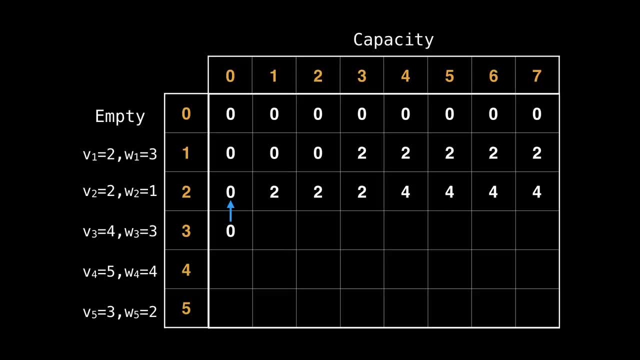 Meaning the cell directly above. so this one, that one, the state also, and now we get to a capacity of three and we are able to improve the best value from two to four. by including item three, we are also able to improve the best value from four to six. 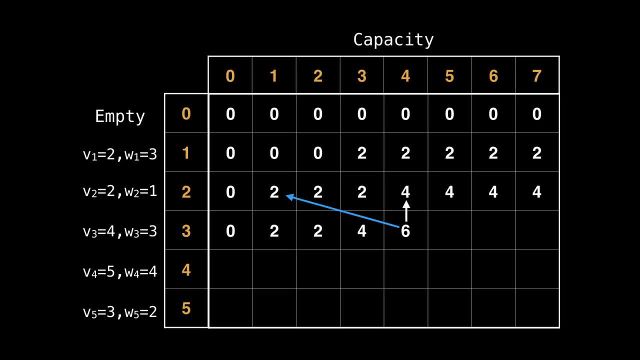 by adding on the value of item three to the cell being pointed to by the blue arrow. A similar procedure is used to fill in the rest of the row and the rest of the matrix. At the end we finish filling the table and we can get the best value of selecting a subset of the 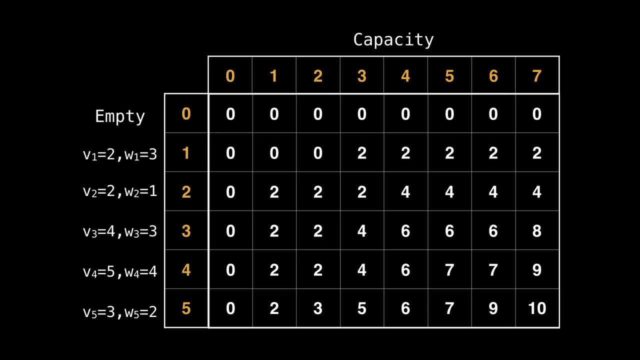 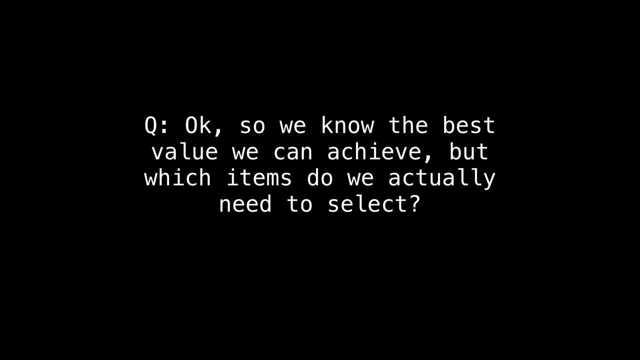 five elements we originally started with. the best value we can get is going to be found at the bottom right corner, which in this case is 10.. Okay, great. So now we know how to achieve the best possible value, But we still don't know how to actually select the. 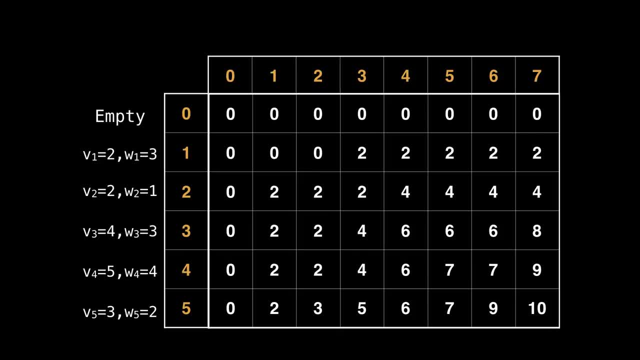 correct elements. To do this, the idea is going to be to start at the bottom right corner and work backwards. We include an element if the current value and the value in the row above it differ, The idea being that if the two values differ, then the row we're. 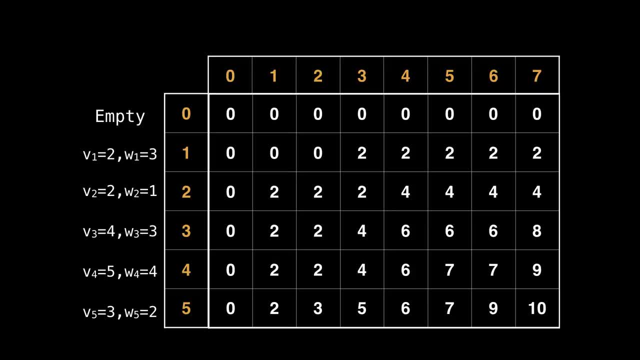 currently on must have a value of 10.. And if the two values differ, then the row we're currently on must have a value of 10.. And if the two values differ, then the row we're currently on must have had its item included. Otherwise, the value would not have changed. Let's see an 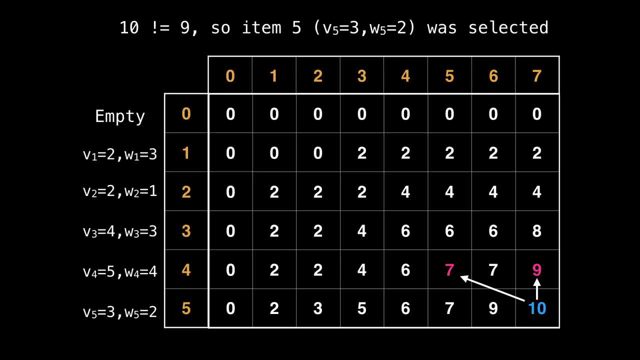 example of this. So we start at the value 10 at the bottom right corner and look at the value directly above, which is nine. nine and 10 differ in value, So we include item five from the last row. Since we included item five, we need to subtract off its weight. 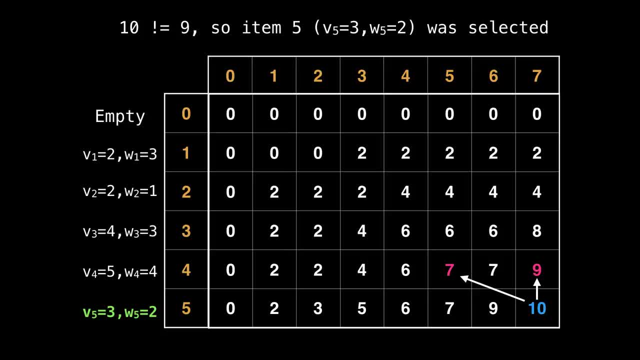 so that we can consider a smaller knapsack size. So in doing this, we're going to have to remove a weight of two and shift our focus to where the diagonal arrow is pointing. Now we're only considering knapsacks of capacity five, Since the value of the current row for 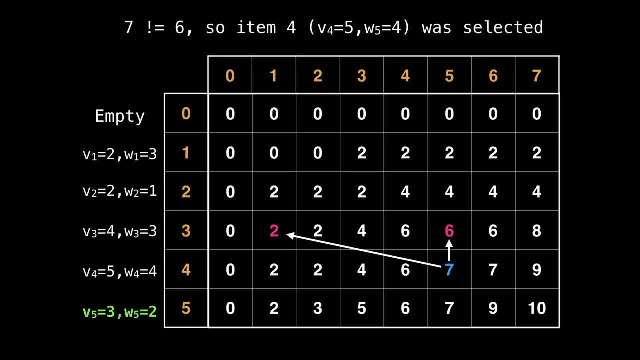 item four is seven and the row above it is six. we know that we also need to include item four, So item four gets included, And yet again we need to reduce our knapsack size And move to where the diagonal arrow is pointing. Now we're on column one, So we're only considering. 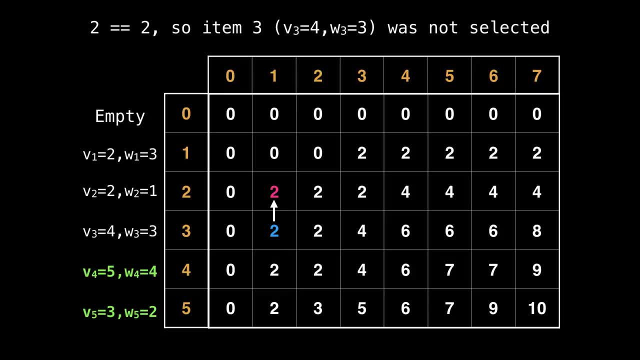 knapsacks of size one. the value of the current row and the row above us are equal, So we do not want to include item three. So we can move up and not change the column. we're still only considering knapsacks of size one. So we check the value and the current row and 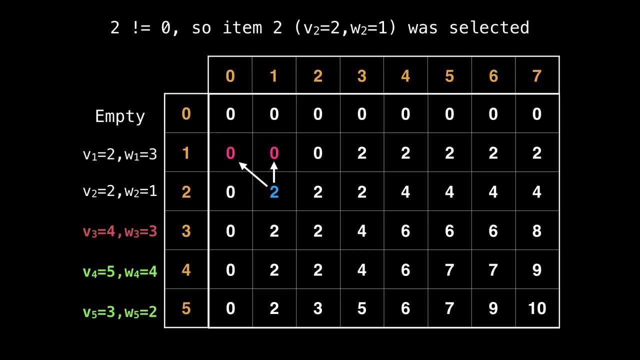 the row above which differ. So we include item 10.. To: the last item does not get included, since zero is equal to zero, meaning that there was no change here. So, in summary, we selected three out of five of our items, those that 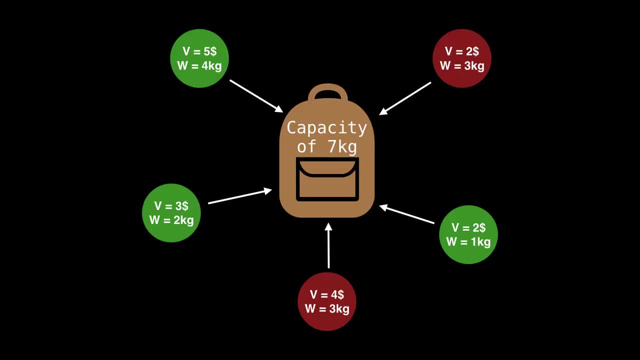 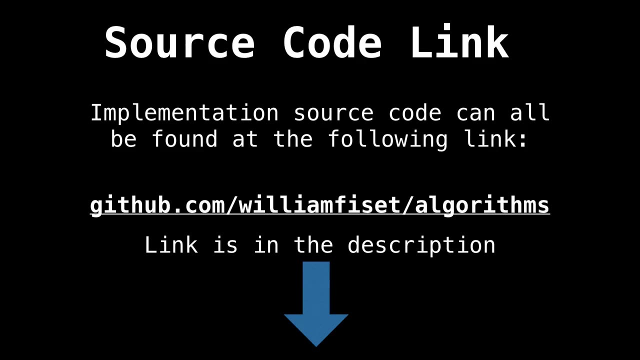 are in green at the moment, that is, the four kilogram item worth $5, the two kilogram item worth $3, and the one kilogram item worth $2.. Now let's look at some source code for the 01 knapsack problem. you can find the source code I'm about to show you at the end. 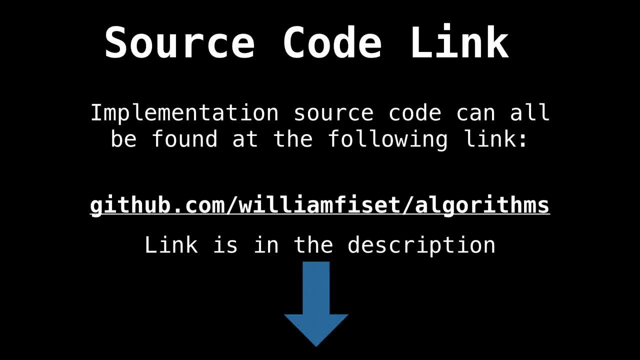 of this video. So I'm going to go ahead and show you how to do that. So I'm going to go ahead and show you how to do that. So I'm going to go ahead and show you at githubcom: slash William physio, slash algorithms, And there should also be a link in the description. 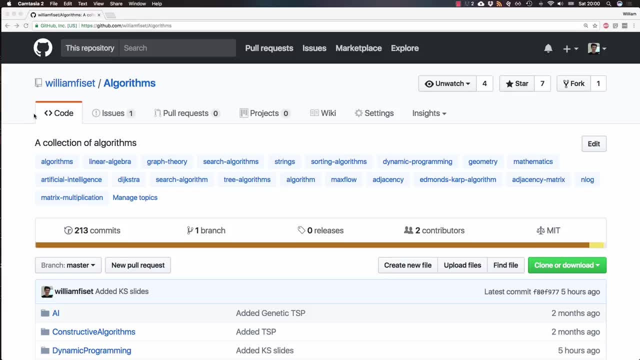 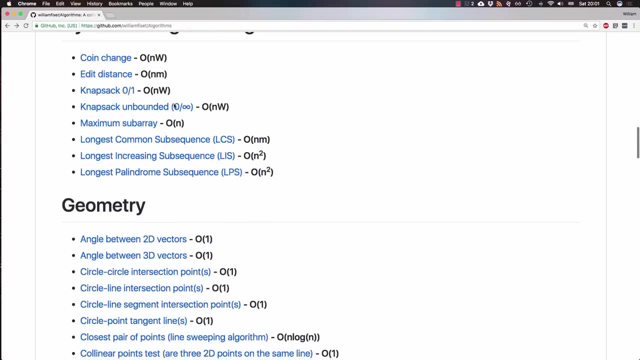 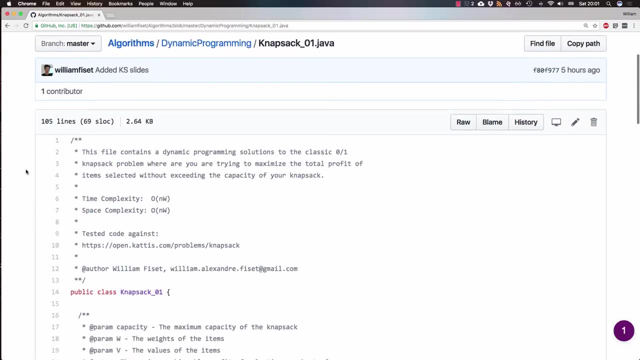 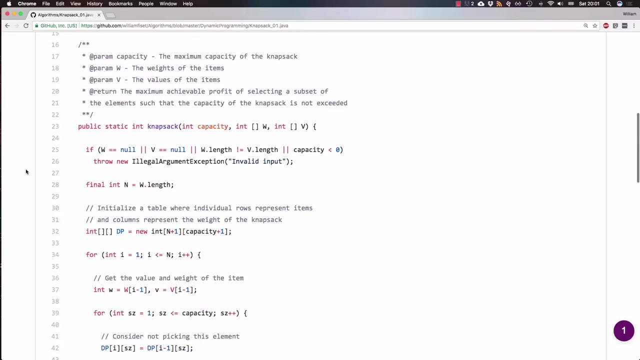 below. So here I am on my algorithms repository And if you just scroll down and go to the dynamic programming section and click the knapsack link, it'll bring you to the knapsack Java file. So if we scroll down to the knapsack method, you can see that it takes three parameters. The first one is the capacity. 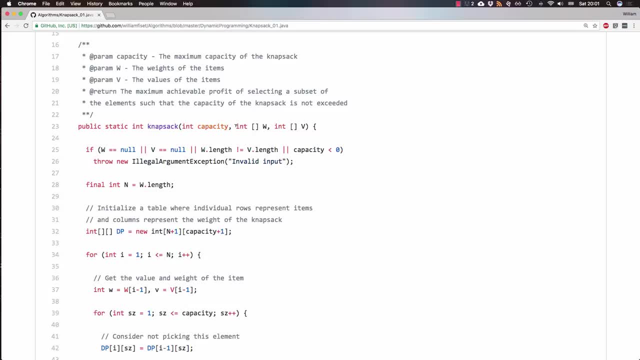 of the knapsack, And then it takes two arrays called w and v. W is the weight of the items And v is the value of the items. So for index i, you would know what the weight would be and what the value would be. 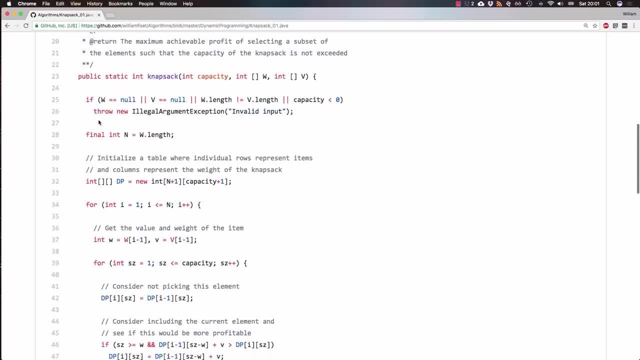 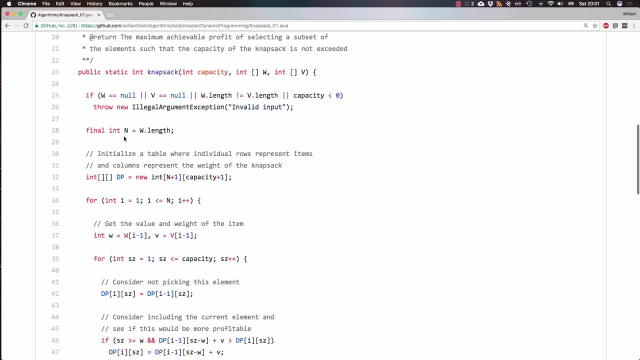 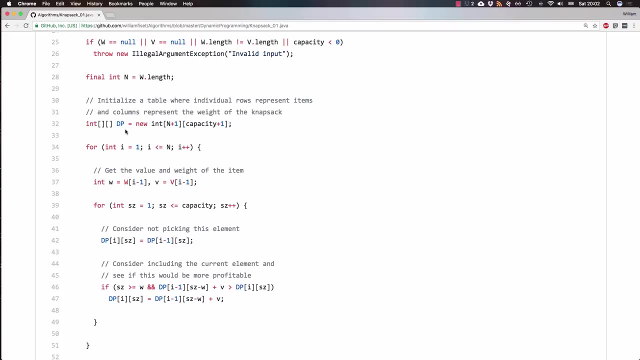 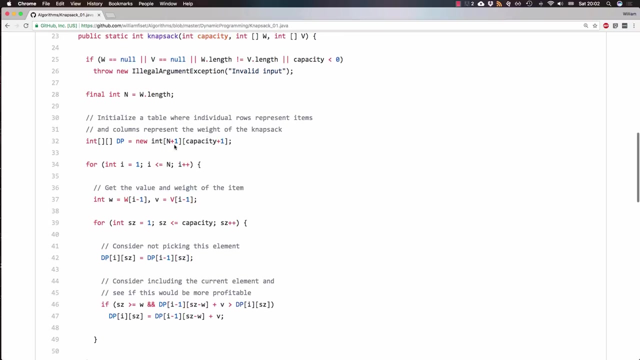 Next, I just do a quick check to validate some input. then I get the number of items passed in, So that will be n. Then I initialize our table, which I call dp for dynamic programming, And I make them 11 larger than we actually need, just for index, out of bounds issues, just so. 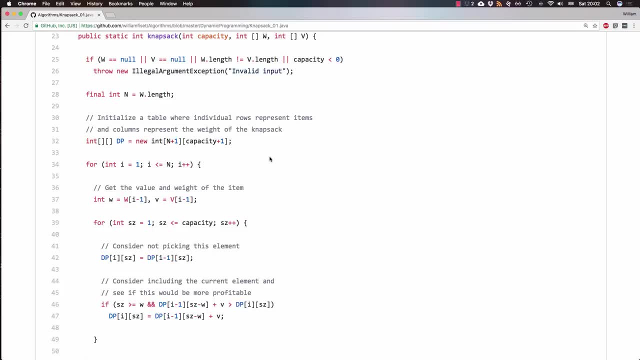 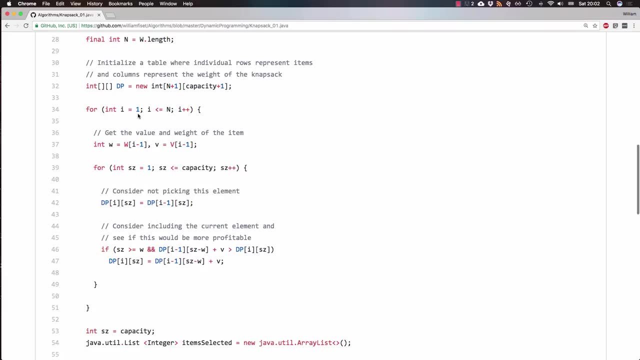 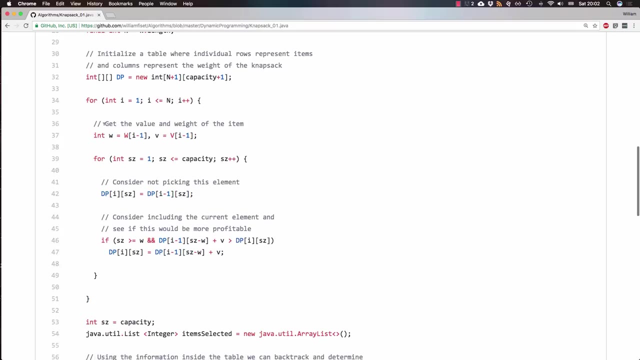 that we can more easily reach into our table. Next, I loop through all our items. Note that this loop is one based, it's not zero based just because we made the table one based. So when I reach in to get the weight w and the 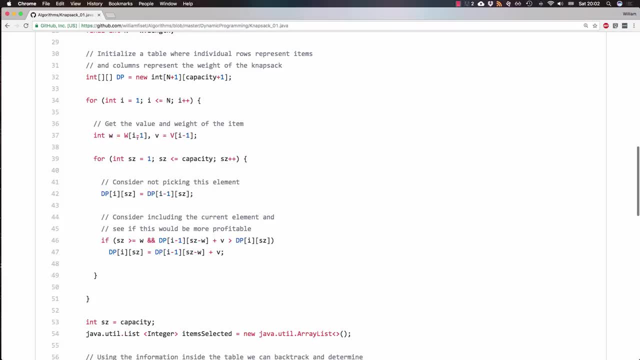 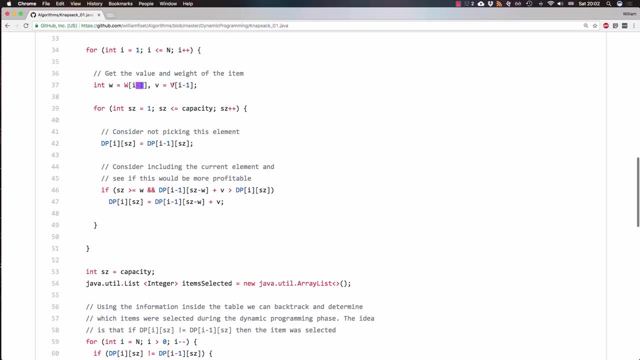 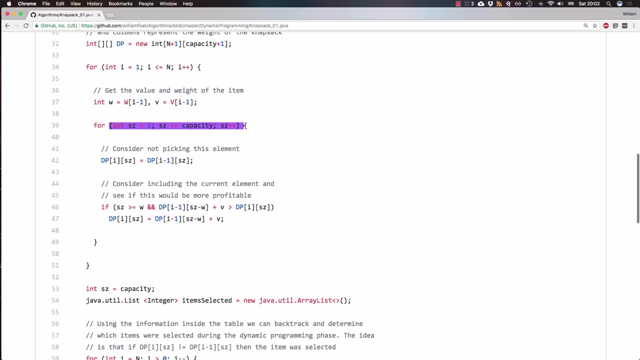 value of our items. since I is one base, I need to shift back one, because the arrays we passed in are zero based. So that's why there's like these minus ones. right here, Just a little detail, And then for each knapsack size, we consider not picking the item. So that's. 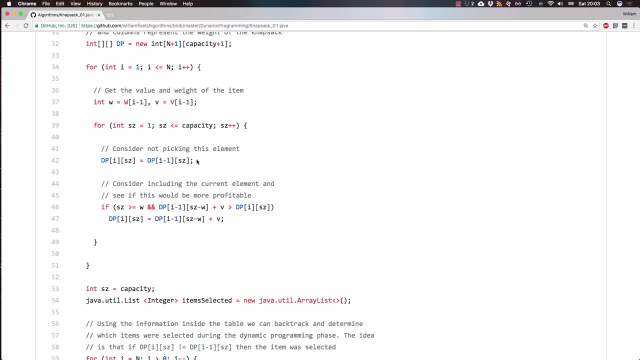 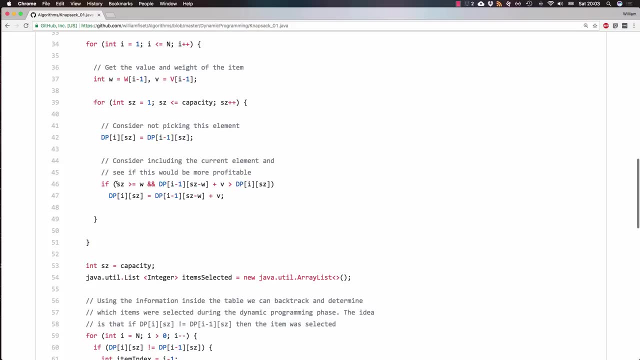 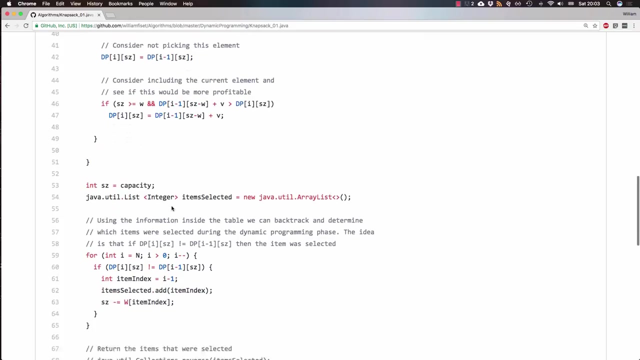 looking at the row directly above us and then initially set that as the best current value And then we check if we can update to a better value by including the current item. So this would be the equivalent of one of those diagonal arrows in the slides Next up. this is an optional step that this whole section just looks. 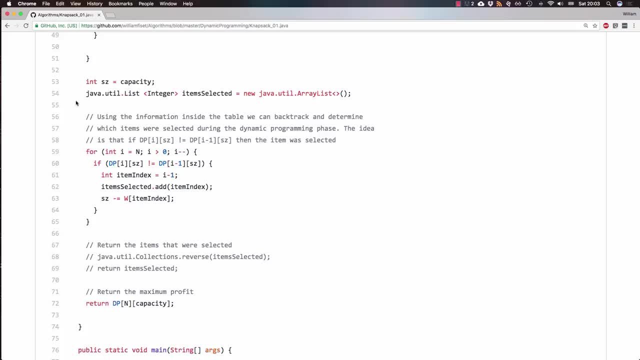 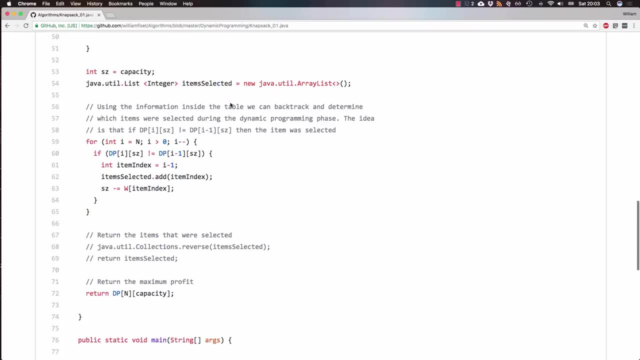 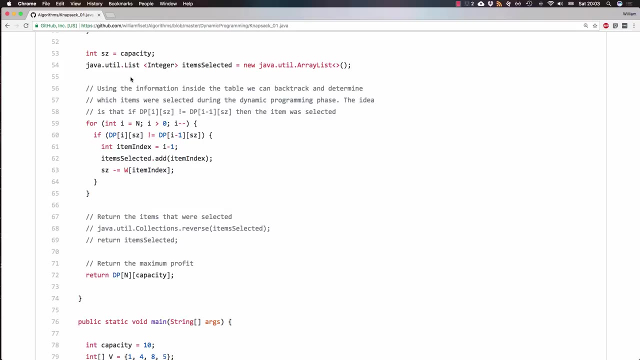 and tries to find what elements were selected. So those get stored inside the items selected array And all I do is I start at that bottom element and then go up and search for the items we need. Let's look at the loop structure. So start i at n and then decrease i. this is the 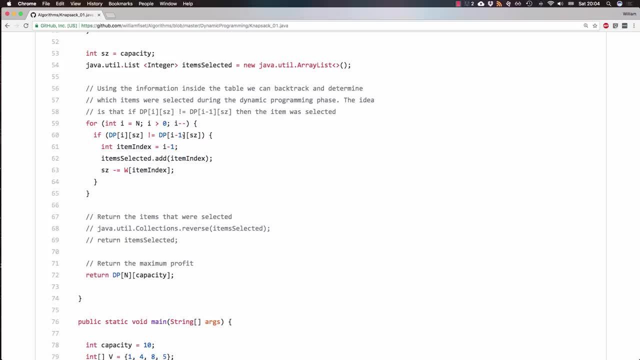 check that looks at the row above to see if there's a mismatch. And if there's a mismatch, we know to include that item Again. my index is one based, So I need to subtract off one and then I can add that.